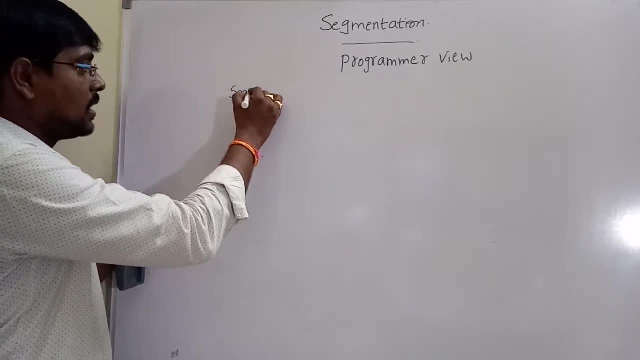 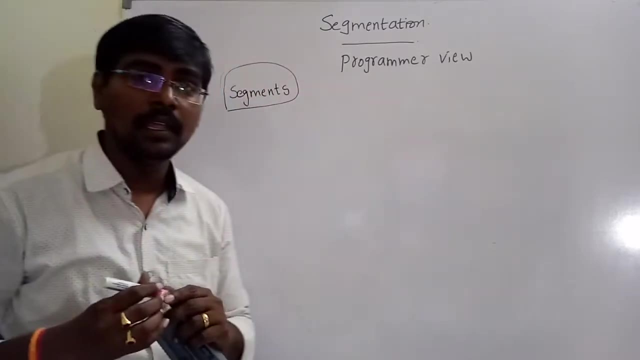 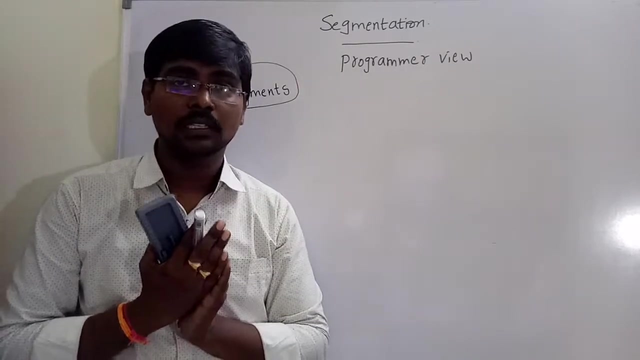 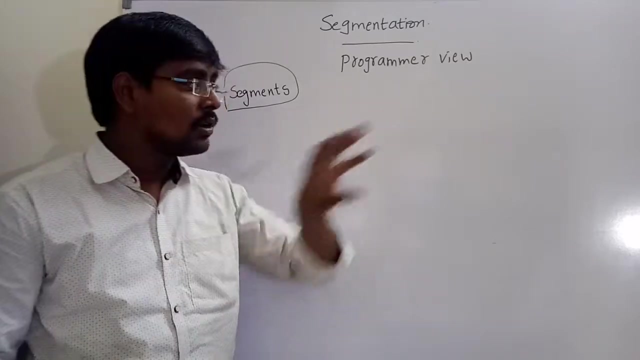 Here the total logical address space is divided into a collection of segments. Logical address space is simply a collection of segments Here in programmer's point of view. some programmers think that the memory is a sequential, that is, an array of linear bytes. One part: we are storing instructions and 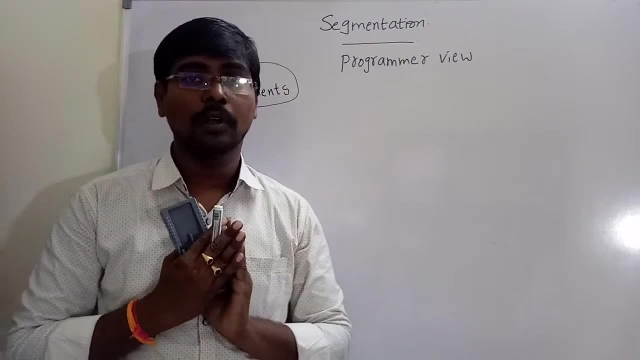 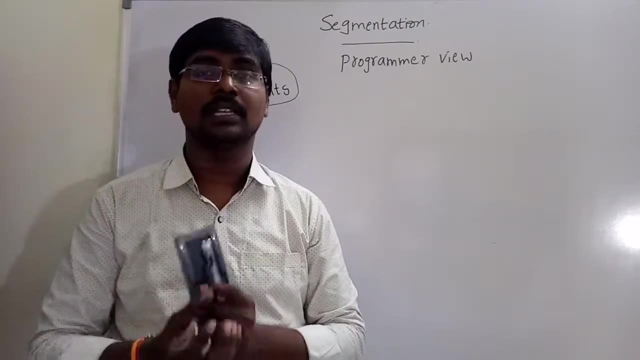 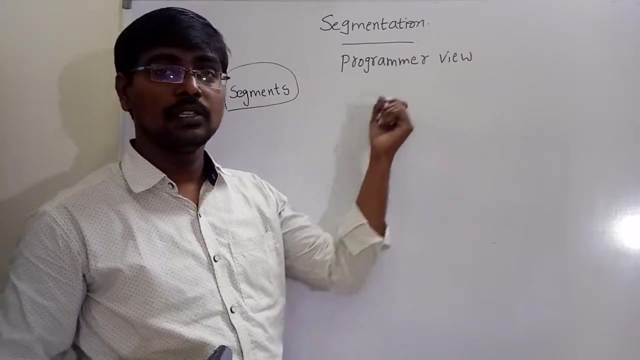 next part. we are storing data. Some programmer's point of view here. some programmer's point of view: the total memory is divided into different number of segments. Here, segment means simply a part Divided into different segments. The information is placed in different segments. 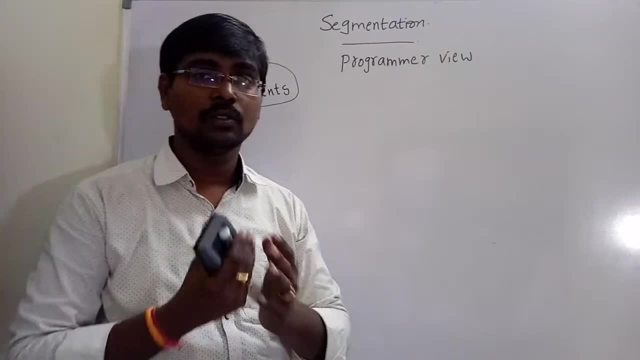 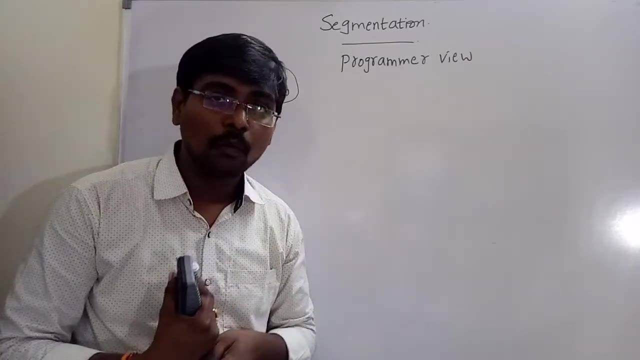 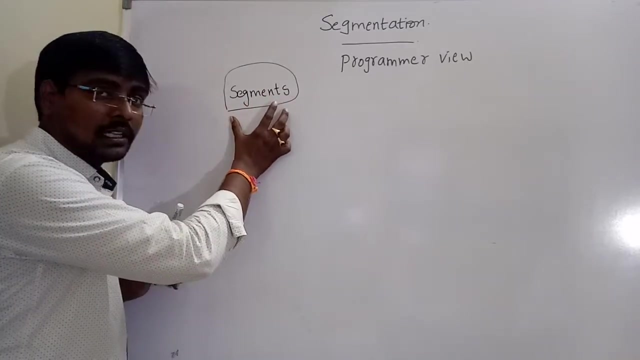 And there is no order. So there is no need of ordering of segments. This is some programmer's point of view. Now we are considering this view. That means in the segmentation the first two things is logical. address space is divided into different number of segments. 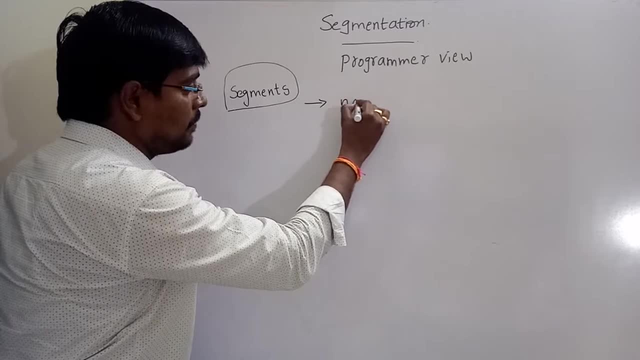 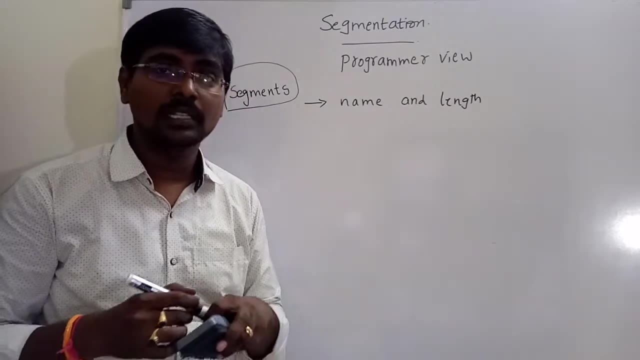 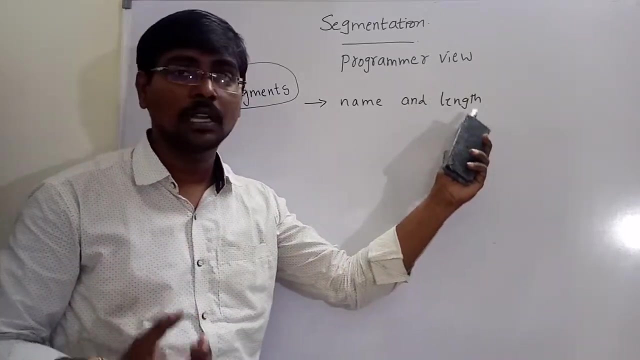 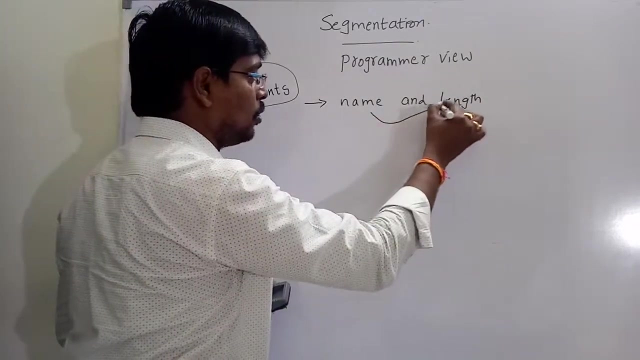 Each segment have name and length. Each segment have name, That is the name of the particular segment, And length specifies how many number of elements or items that are placed in the segment Contains both name and length. That is, by using these two, By using these two attributes, we are accessing a particular segment. 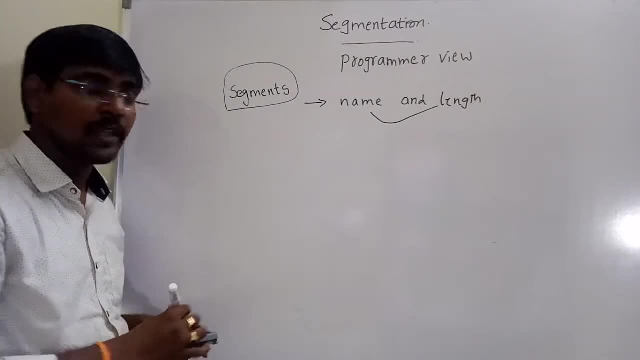 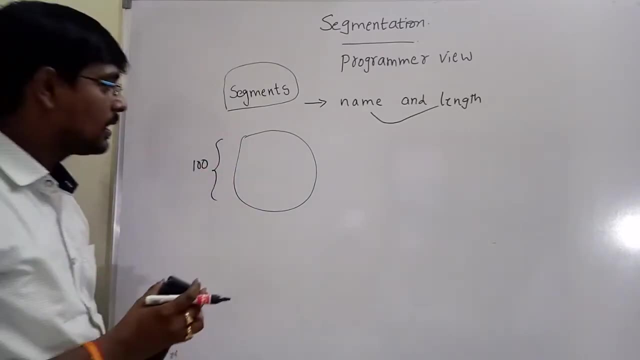 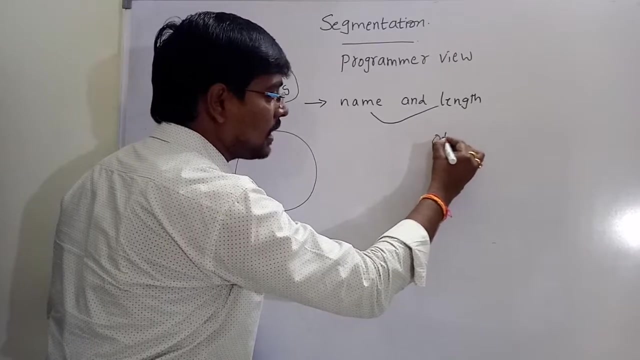 How we are accessing, even though we know the length. For example, this is a segment. The length of the segment is some hundred. That means the segment contains hundred number of elements. How to access a particular element. So a particular element is accessed by using offset. 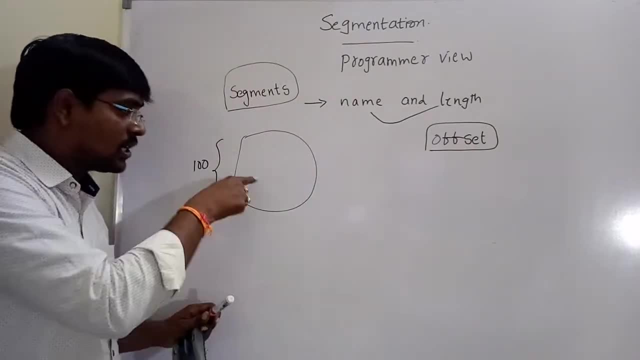 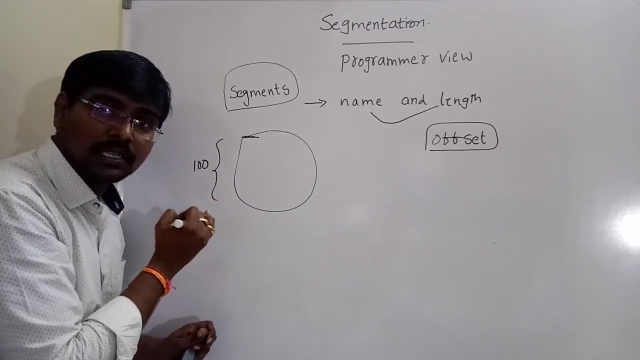 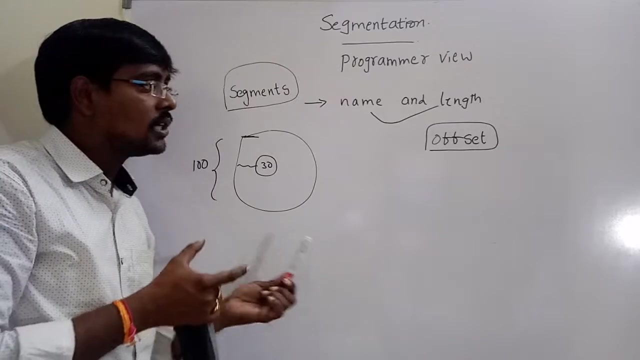 Offset means the distance of that particular element from the base. For example, this is the starting. My offset is some thirty. This is the thirtieth position I am accessing this element, So you got the point. Offset means the distance from zeroth position. 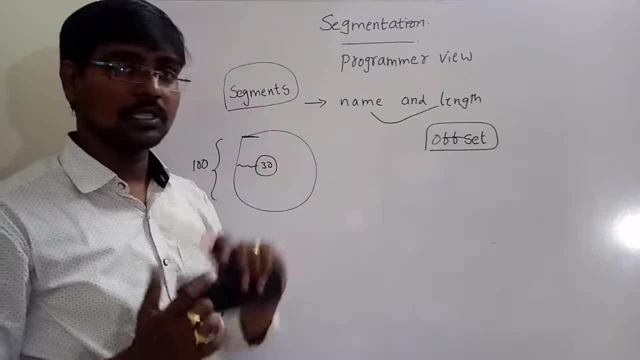 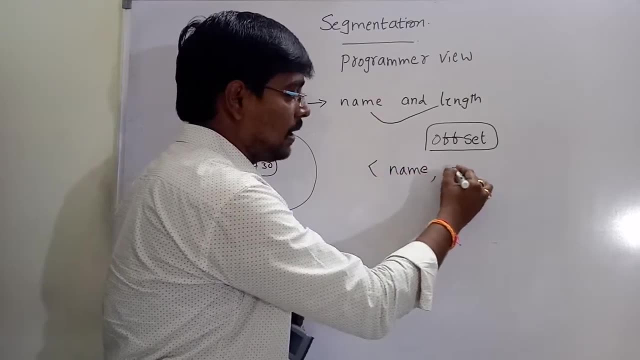 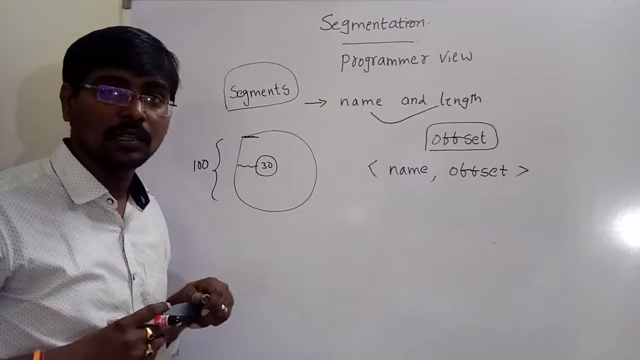 That is the starting of the segment to up to this one. Now how we are accessing the elements? We are accessing the elements by using name and offset. By using segment name and offset, we are accessing the elements from the segment To make our implementation simple. 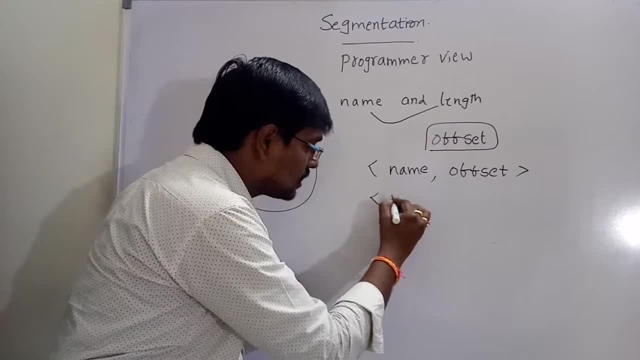 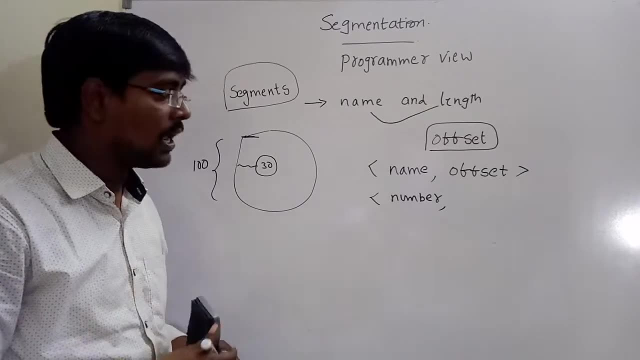 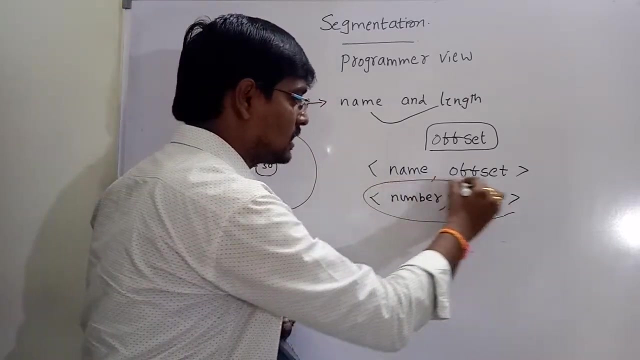 that is to simplify. I am using segment number. Suppose names may lead to conflict. Name may leads to conflict. That's why I am using numbering concept, Segment number and offset. By using this Number and offset, We are accessing the segments. 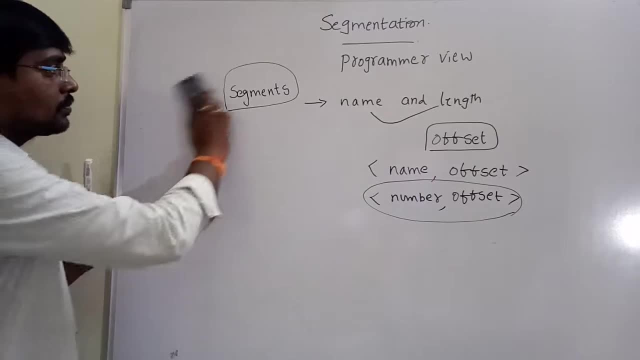 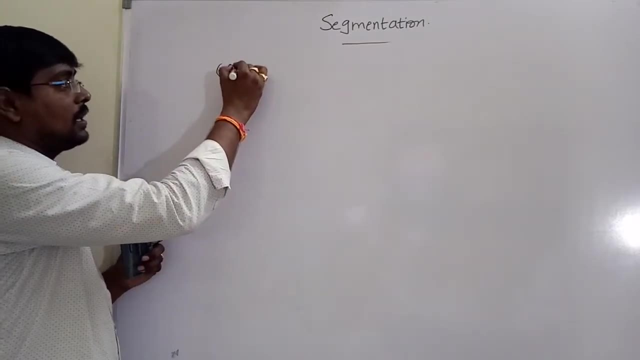 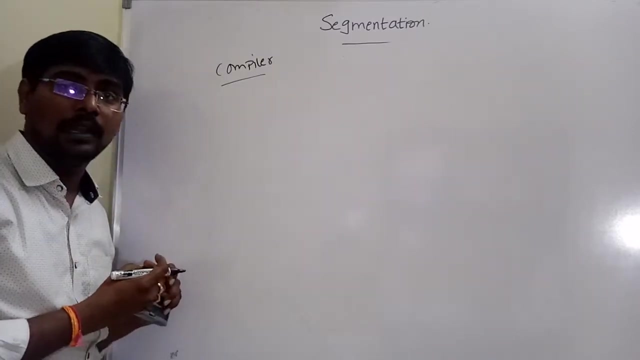 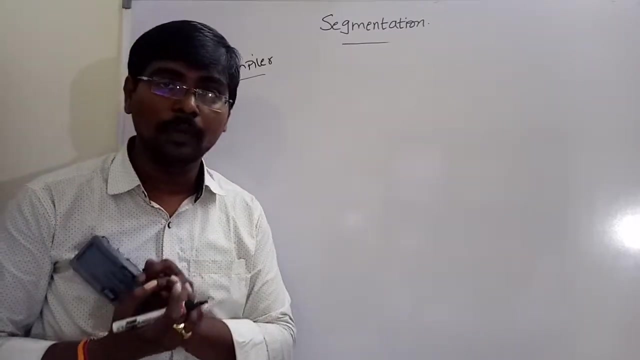 We are accessing the segments. How, For example, For example, A compiler. Consider a compiler Whenever a program is compiled. Whenever a program is compiled, The compiler divides the program into different number of segments, Divides the program into different number of segments. 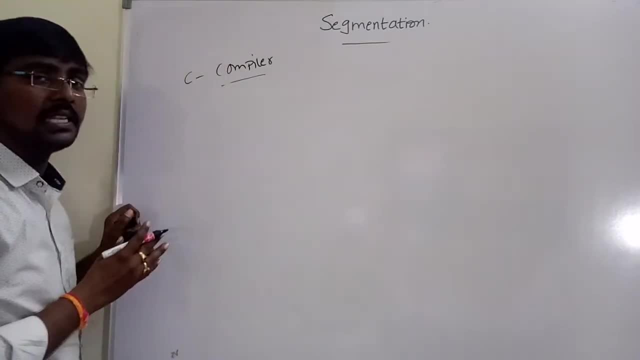 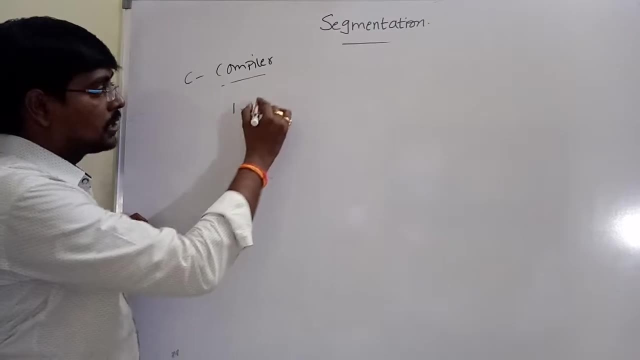 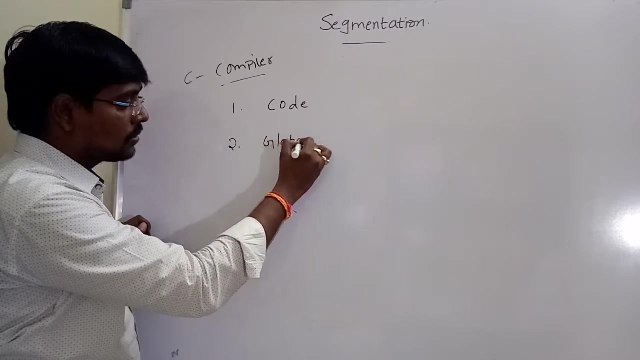 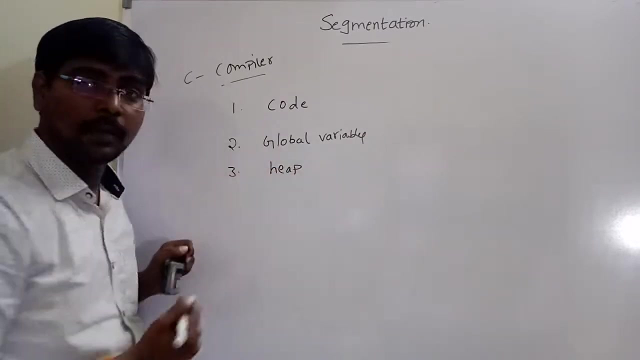 For example, Assume a C compiler, How divide the particular program into different segments? Segment number one, For example: All the code is present in one segment: Global variables. Global variables Present in another segment, Heap. Heap means the memory. 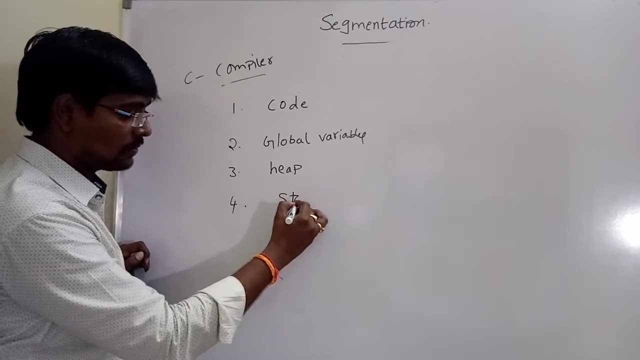 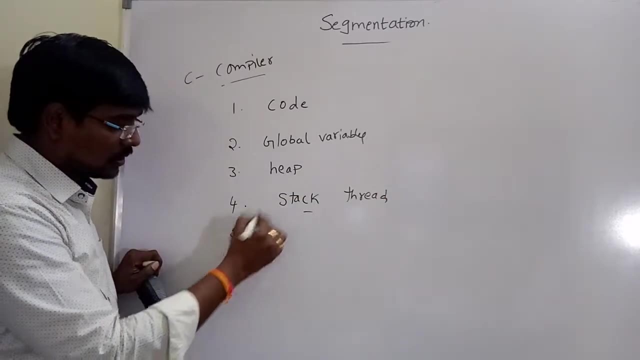 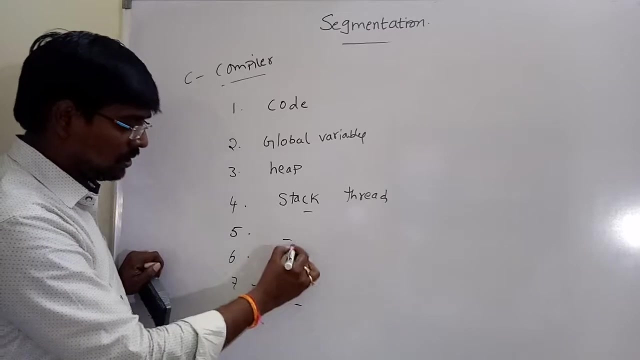 Memory is placed in one segment: Stack. The stacks are used by threads. Stacks are used by thread And Supposing any other thing, Suppose the code: Global variables, Heap, Stack. So in this fashion There is no fixed way. 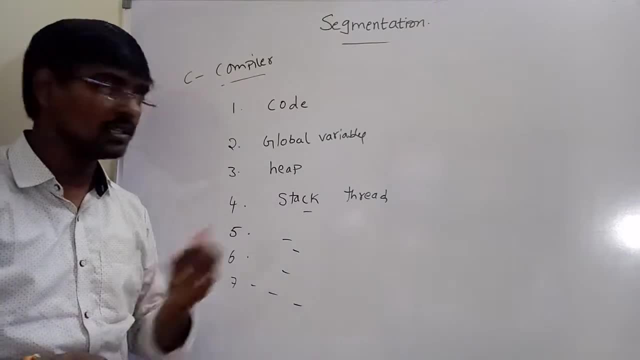 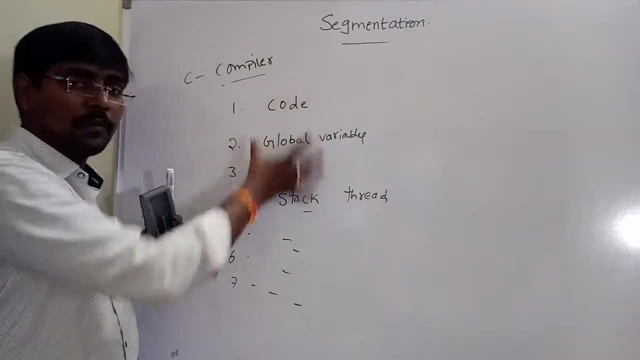 There is no need to. all the code in one segment, All global variables in segment, All heap, All stack. Suppose this is the different way We are dividing our program into different segments. Okay, This is completed. Now Come to the point. 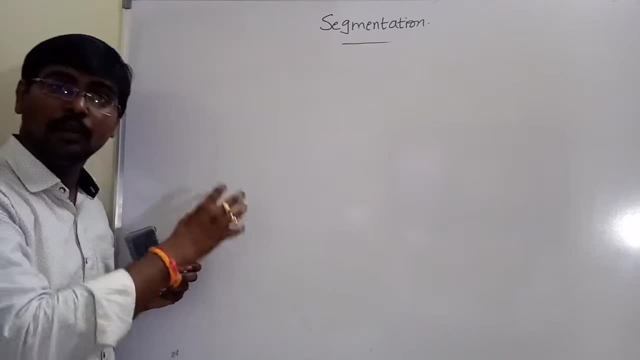 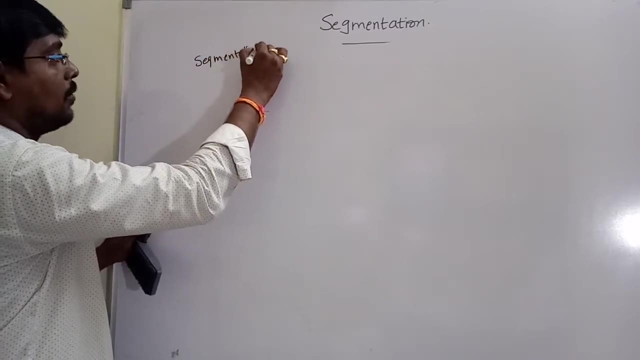 So First point is: Divide our program into different segments. Clear Now Segmentation Hardware. What is the meaning? What we will discuss in this term is: Okay To refer any object. To refer any object, How we are referring. 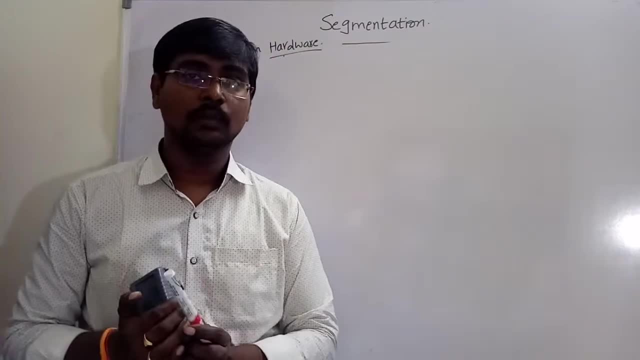 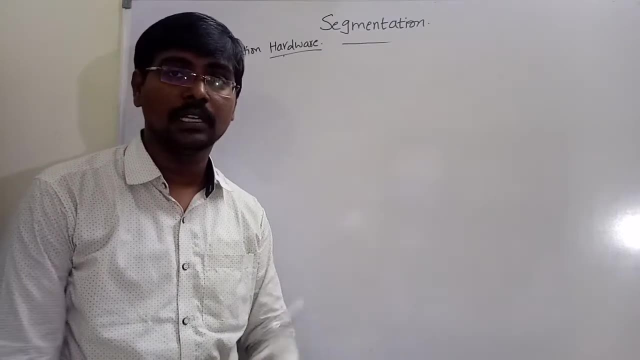 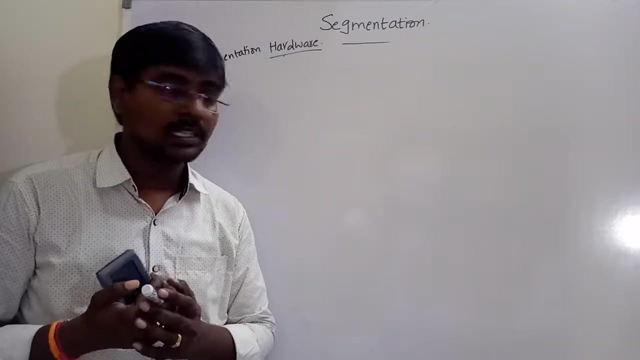 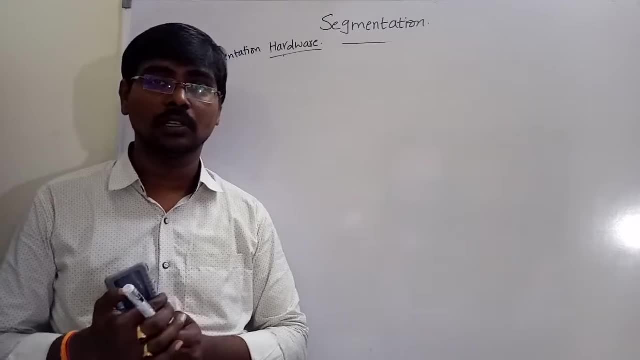 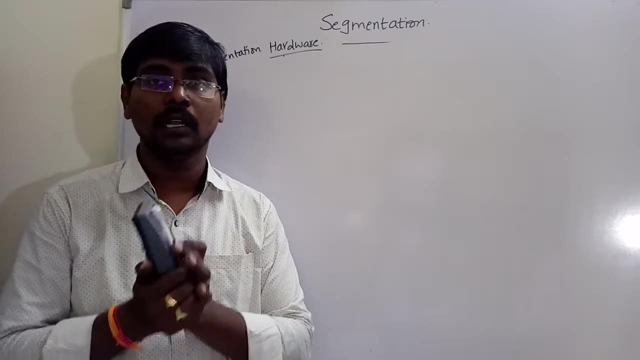 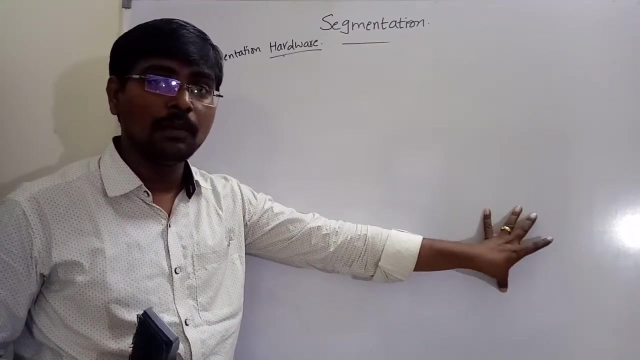 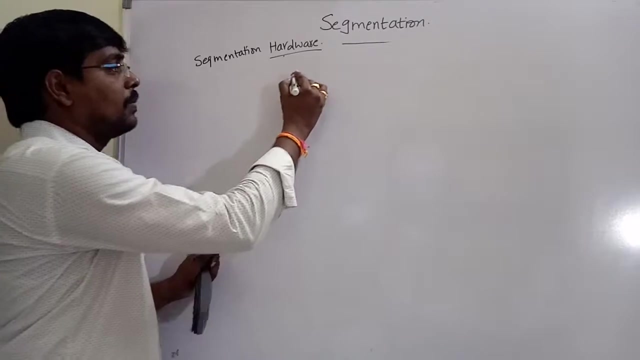 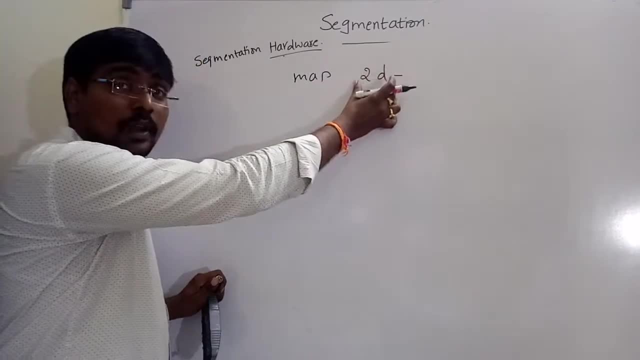 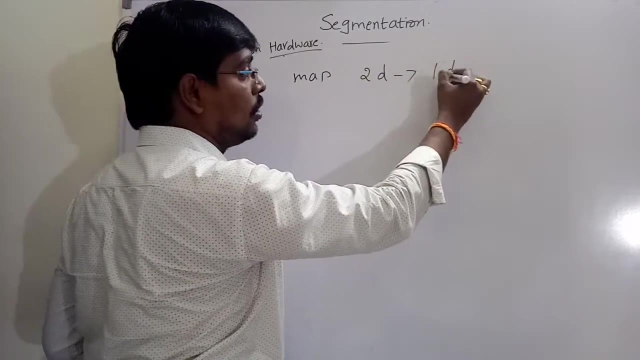 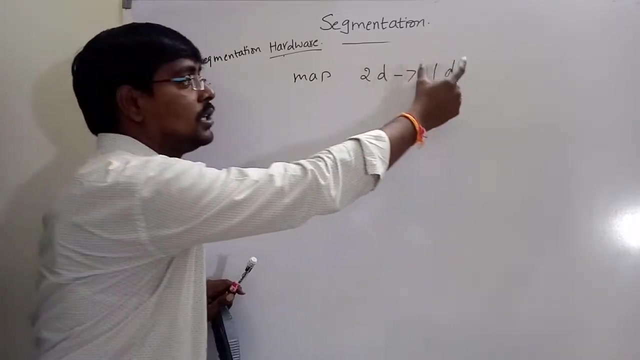 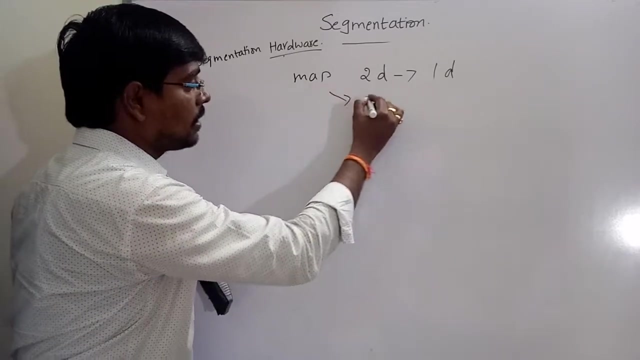 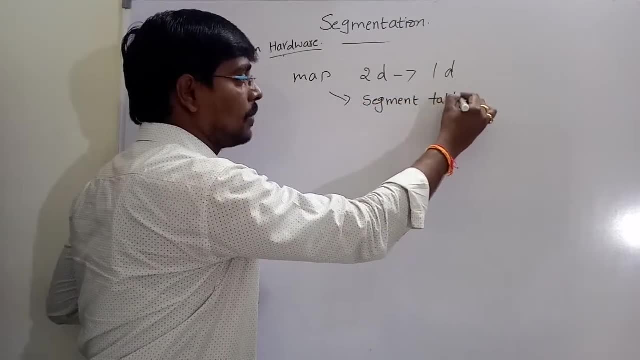 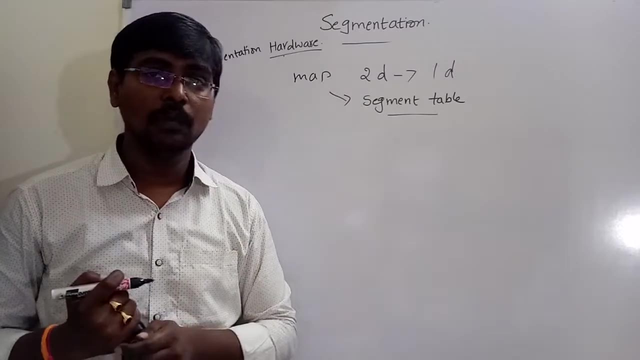 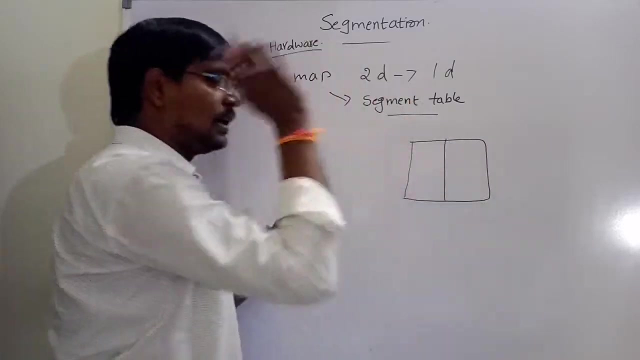 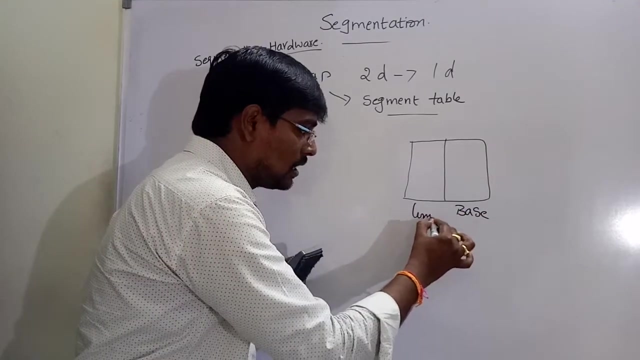 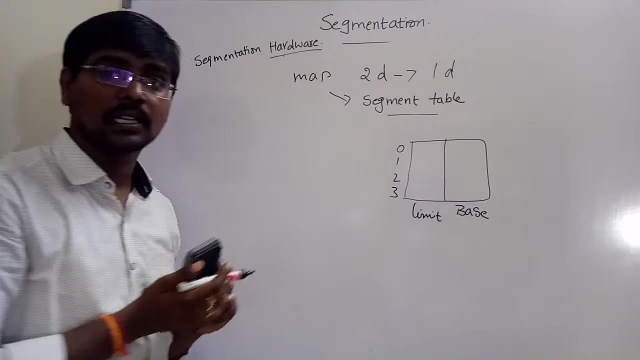 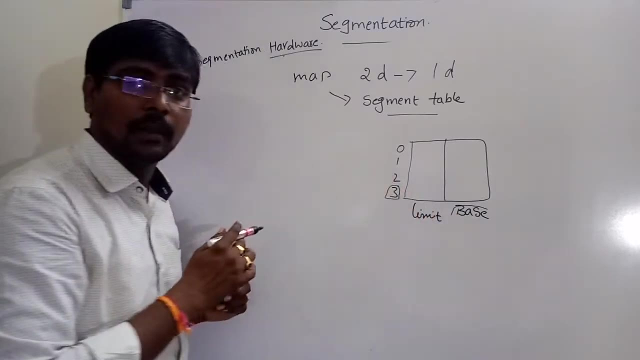 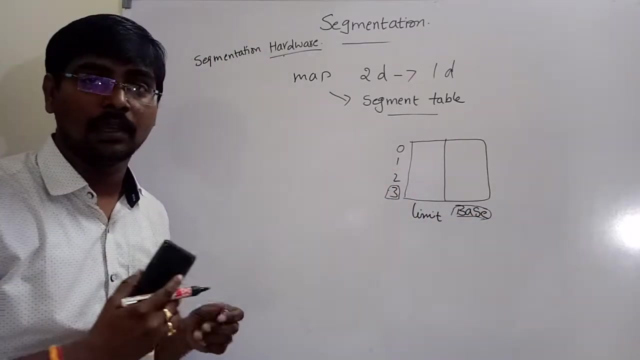 Suppose these are the segment numbers. These are the segment numbers. That means the particular segment. For example, assume segment number 3. Base means the starting, What is the starting address of this particular segment in the memory Base. specifies the starting address of this particular segment in the physical memory. 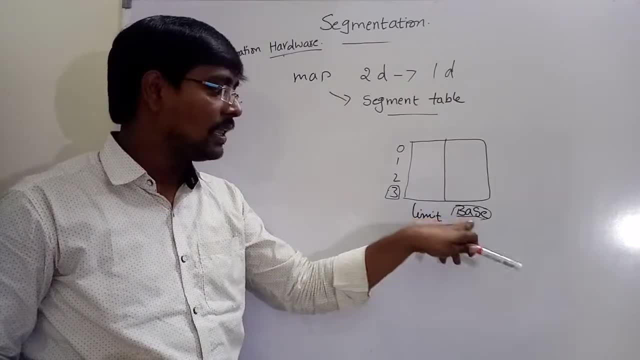 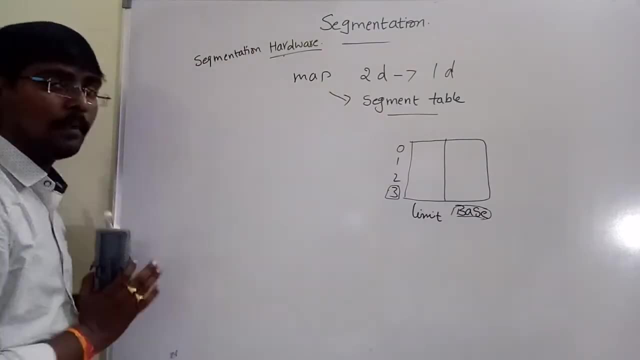 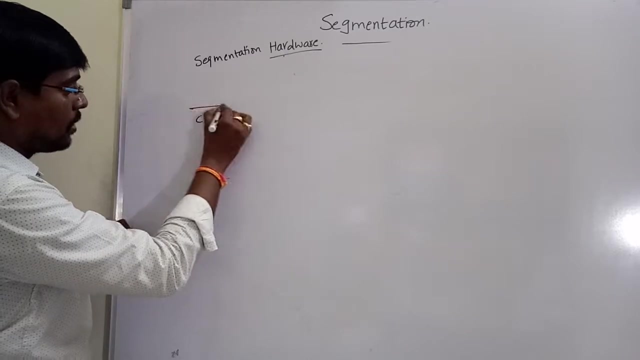 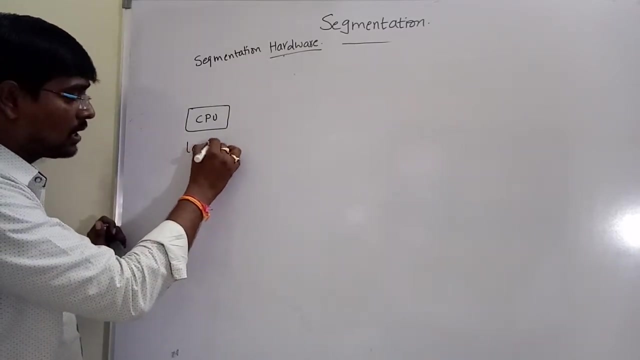 Limit means. Limit means the length of that particular segment from the base, The length of the particular segment from the base. Now how the mapping is performed, We will show with diagram. This is the CPU. CPU generates which address We already know. the address generated by the CPU is called logical address. 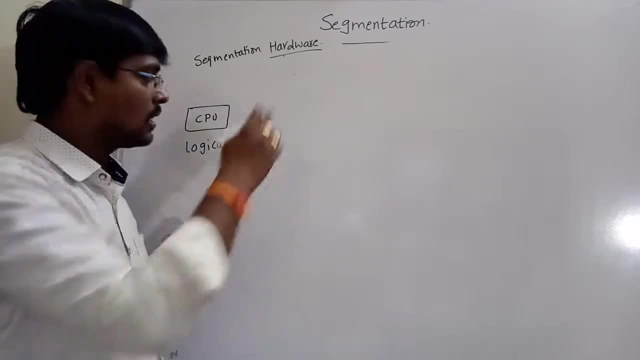 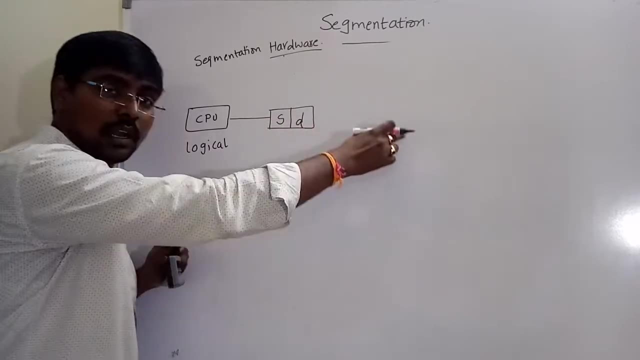 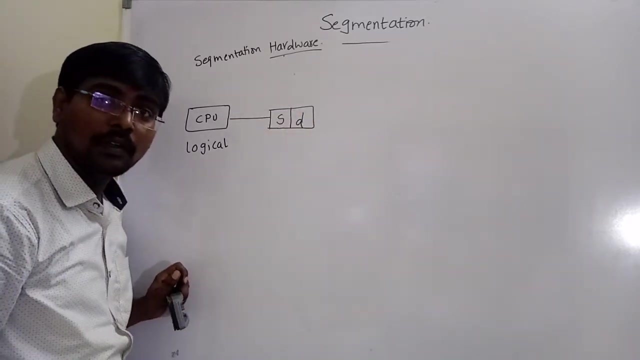 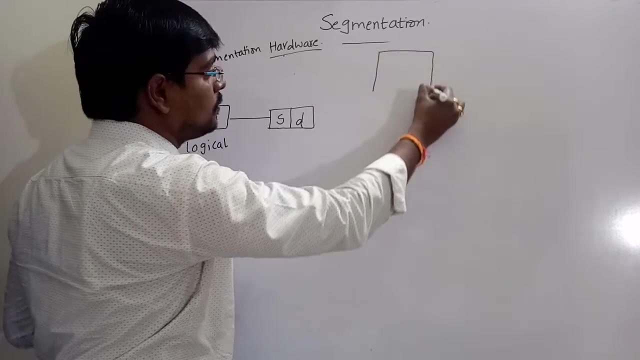 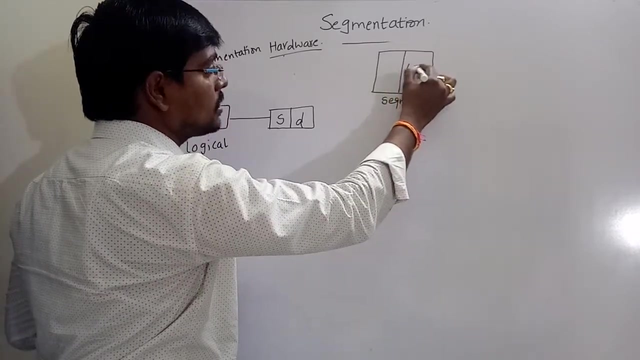 The address generated by the CPU is called logical address. Generates, Generates, Generates Segment number and offset. We already said that We are accessing by using segment number and offset. Now what happens Whenever a segment number is given? This is the segment table. Assume This is a segment table Contains two parts. 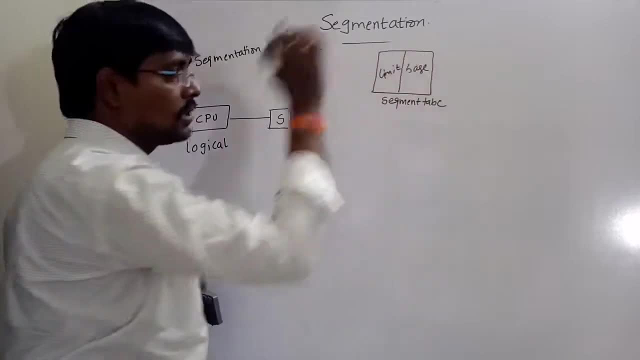 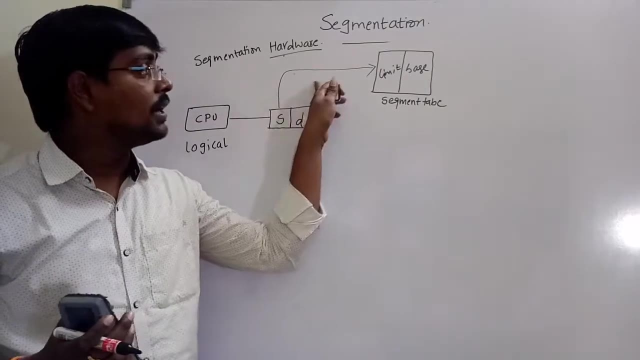 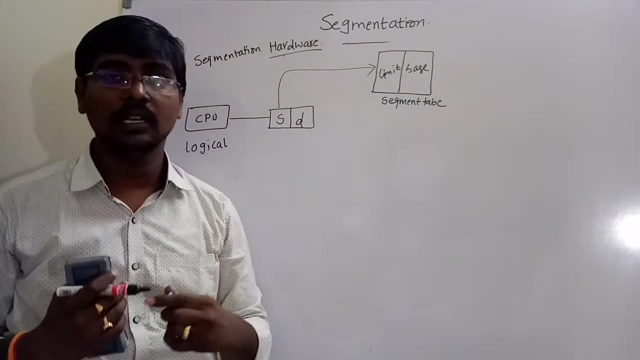 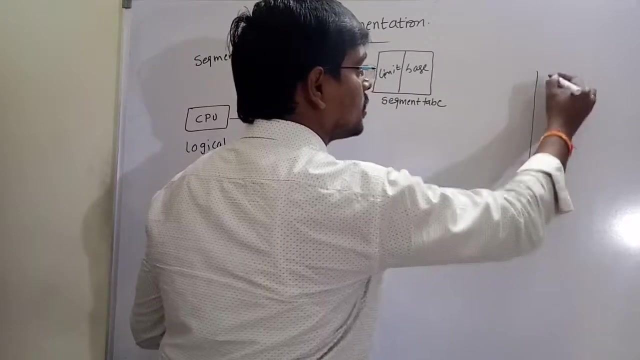 Suppose the first part is base, Another part is limit. Now this segment Segment number is checked into the segment table. The segment number is checked into the segment table. What happens? It identifies the starting address of that particular segment. By mapping by this one, We are identifying the starting address of the physical memory. 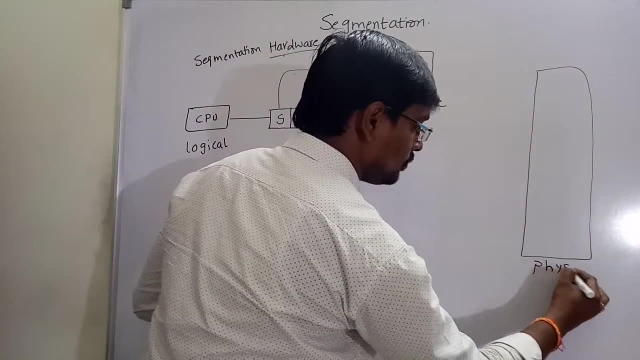 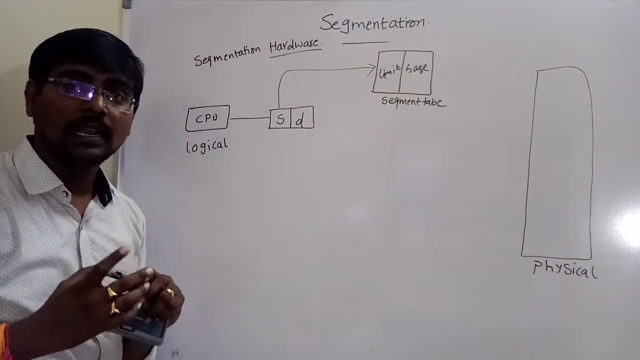 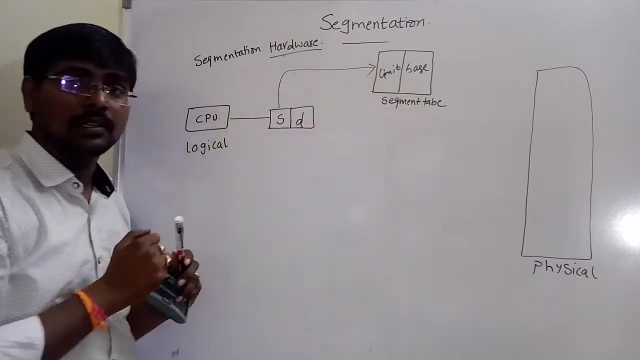 Suppose this is the physical memory. But you have to remember one point Here: limit Limit specifies the length of the segment number, In this case the length of the particular segment Compulsory. this offset is less than this limit. For example, limit is 100. Base address is assume. 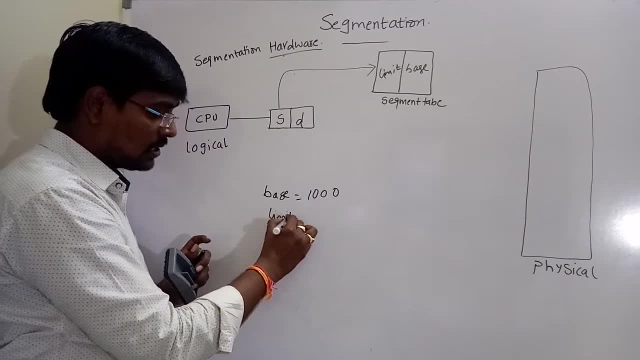 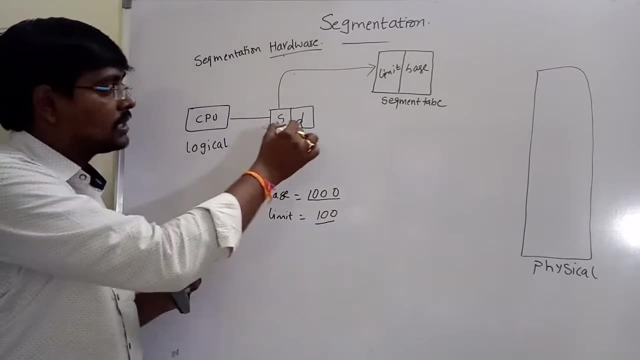 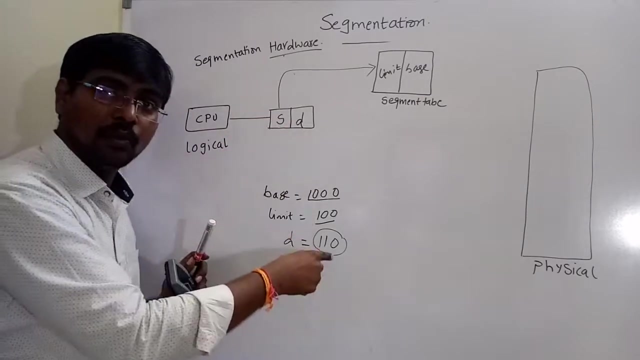 Base address is 1000. Limit is 100, That is, it allocates from 1000 to 1100 only. For example, my offset d is equal to 110. What happens In that particular segment? I want to set the element at position 110, But I have element only at position 100 only. 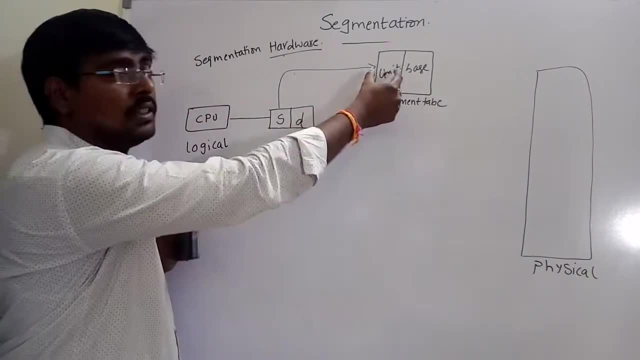 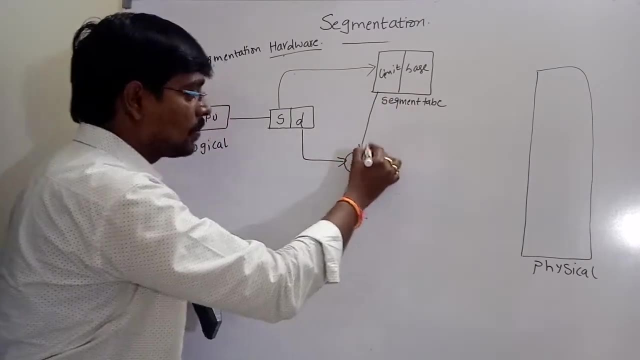 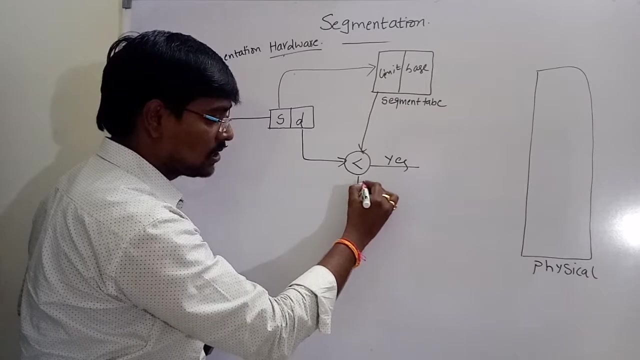 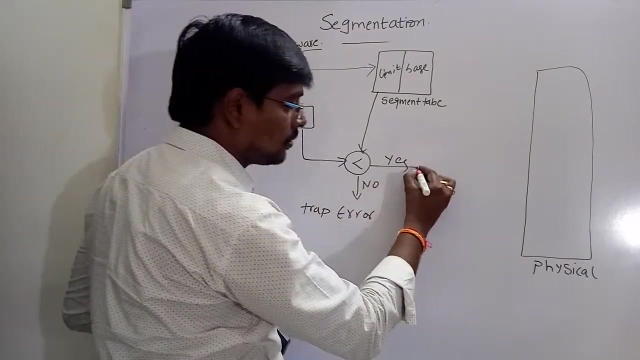 That means Our offset value is within the limit We have to check. Suppose I am checking The condition. Suppose if my offset value is less than this limit, S Suppose the condition false. Simply an error. Simply, it traps an error. If it is yes, Then what we will do? 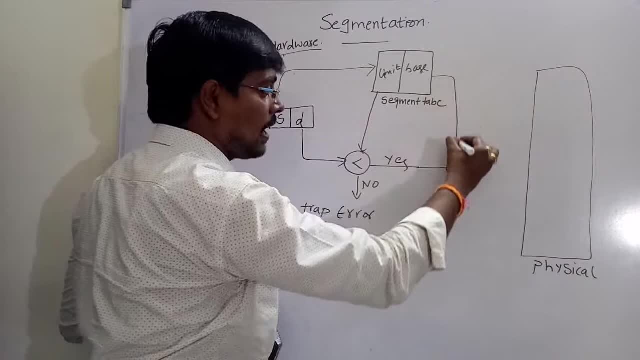 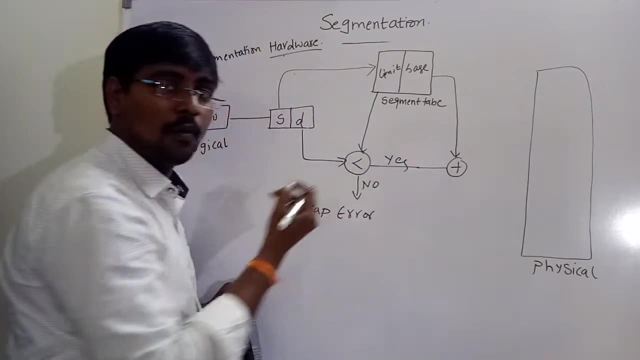 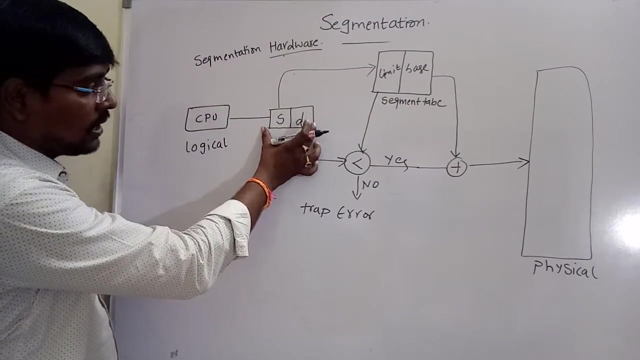 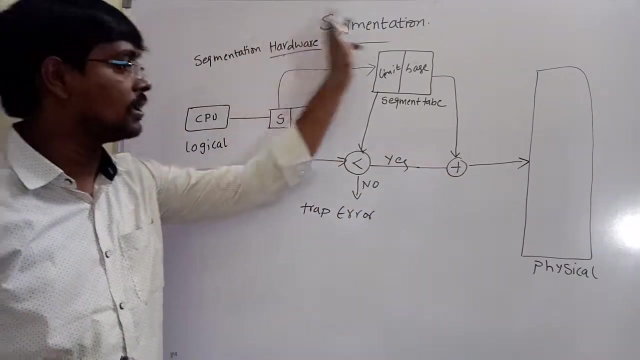 This offset is added to this particular base address. So the starting address and the corresponding offset are added. We are getting one address That is checked in the physical memory. See this one. This two dimensional address is converted into one dimensional. Two dimensional address is converted into one dimensional. 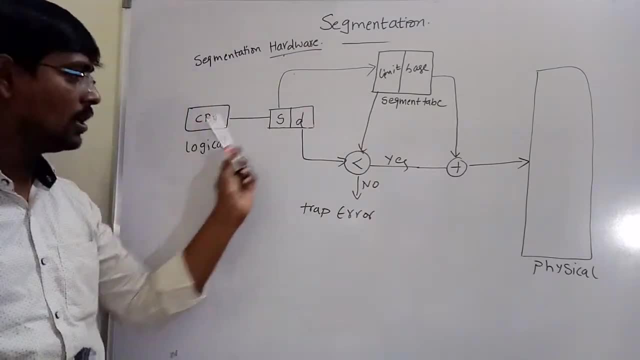 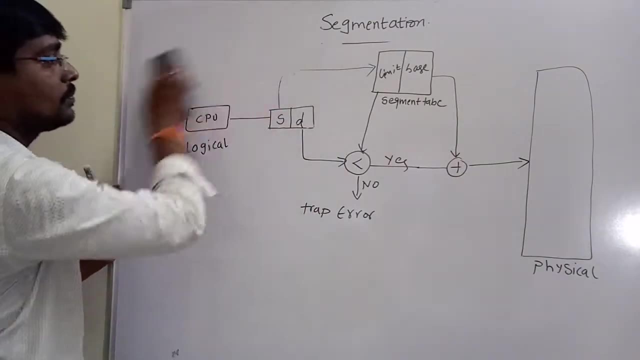 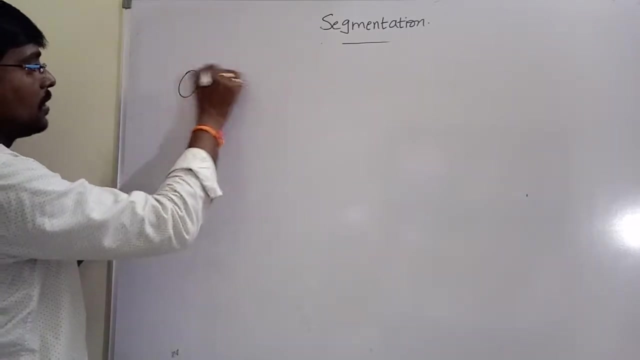 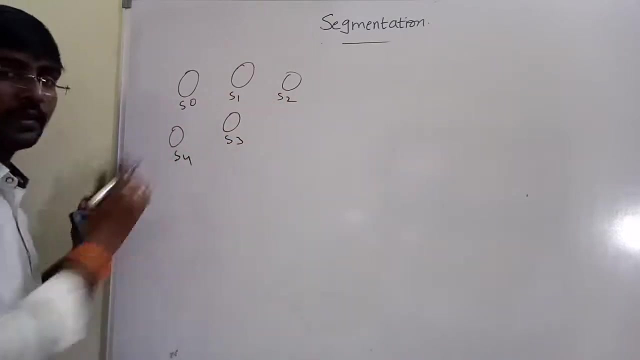 This is the segmentation hardware. By using this procedure, We are identifying the particular segment in the segment table. Now consider an example. For example, we have different segments, Whatever the values present- S0, S1,, S2,, S3, S4. Whatever the values, Maintain a segment table. 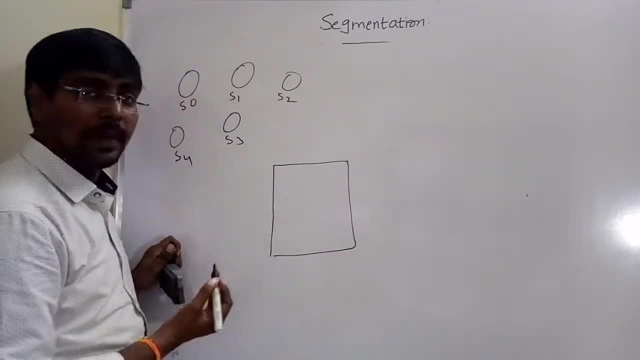 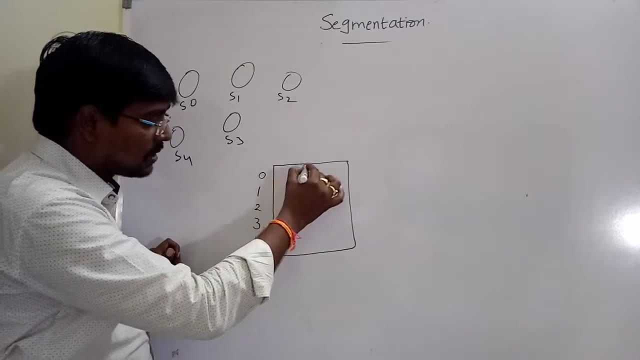 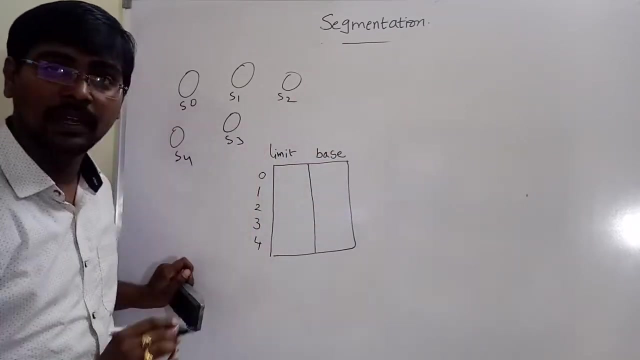 Example is very simple. Maintains a segment table. Suppose 0,, 1,, 2,, 3,, 4. These are the segment numbers. Segment table contains how many parts. Two parts: One part is limit, Another part is base Limit, another part is base. 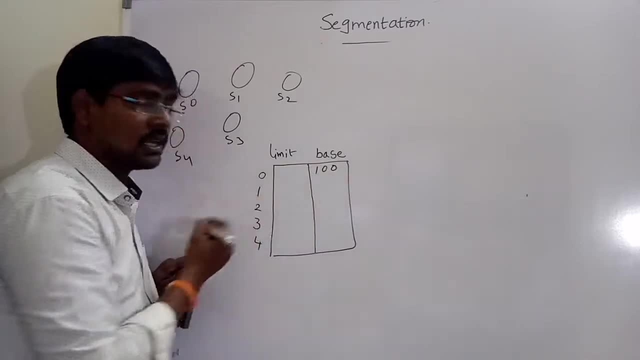 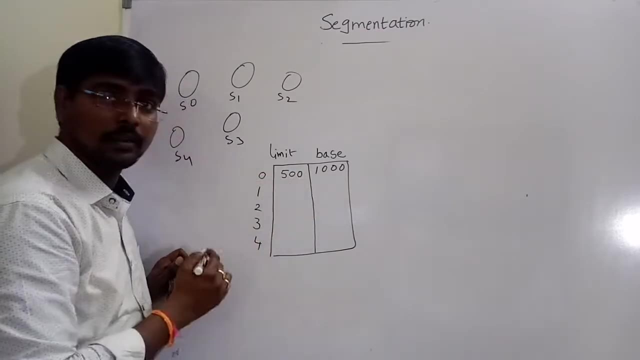 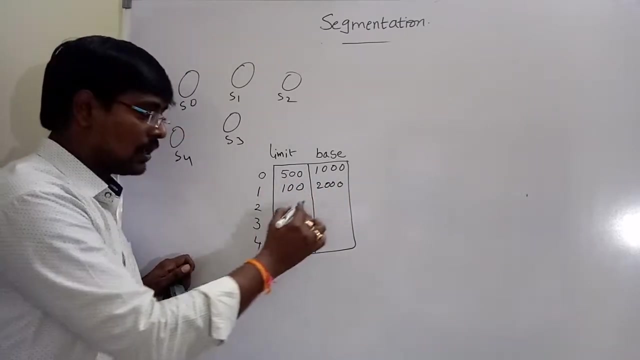 For example, the base address is 1000, The base address is 1000. Limit means, For example, limit is 500, The base address is some 2000. Limit is only 1000. Limit is only 100, The base address is some 2500. 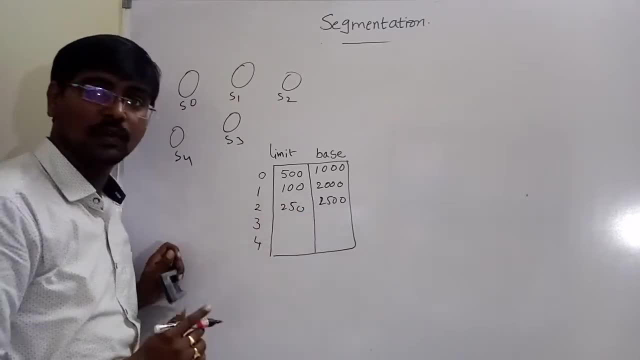 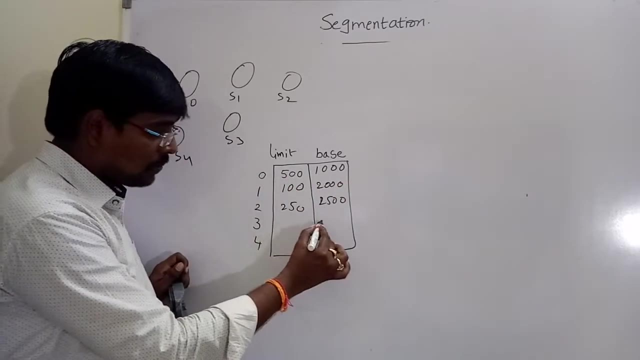 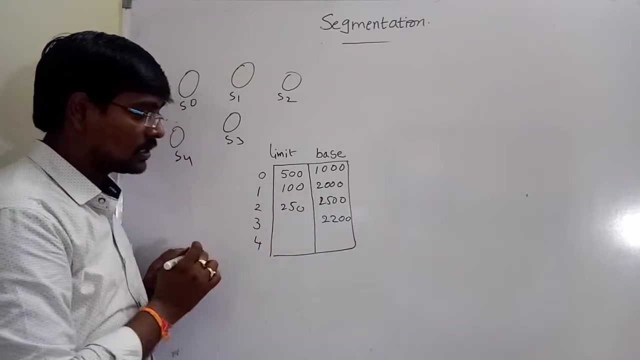 Limit is some 250. In this fashion we are writing: Suppose whatever you are required, Suppose this is some base address, This is some limit. For example, here I am writing: my base address is 2200. Here the segments are overlapped. For example, if this size is 300. 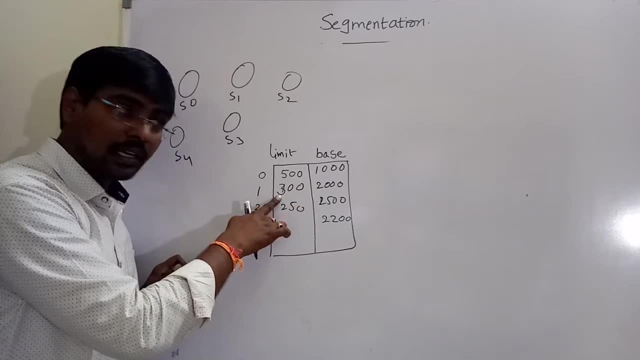 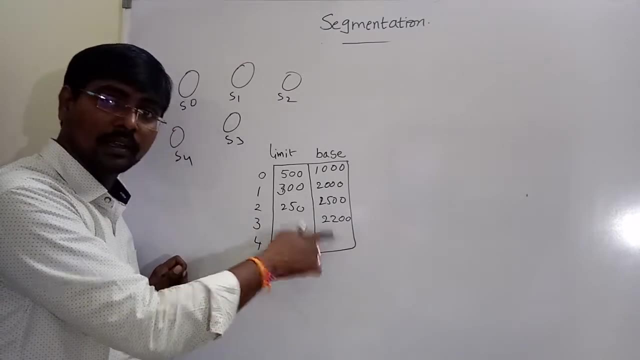 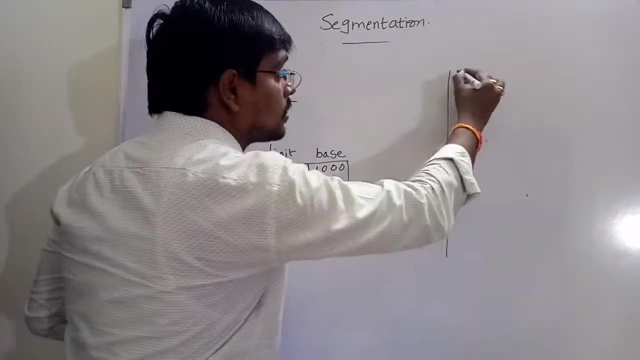 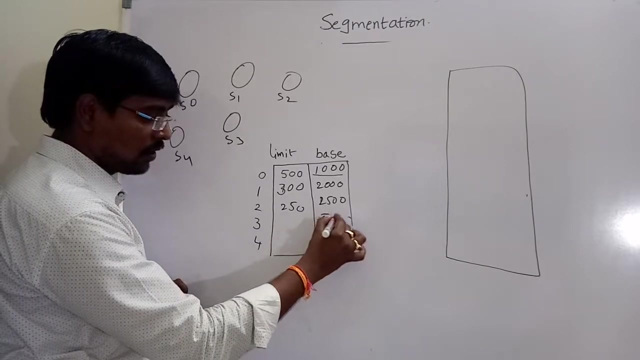 From 200 to 3, That is, 2300 is occupied by segment 1, But I am not mentioning 2200, So it needs to be error Write another. So wow, Suppose this is the physical memory At address 1000. Suppose I have some values also 500. 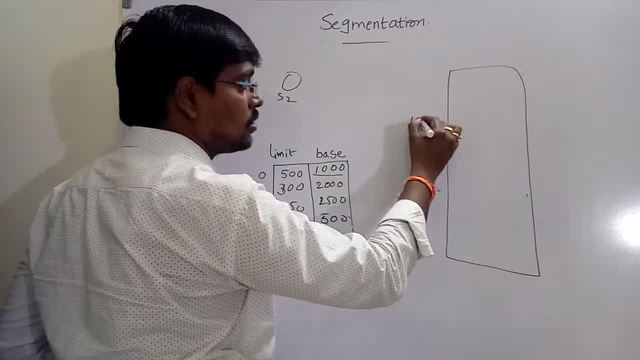 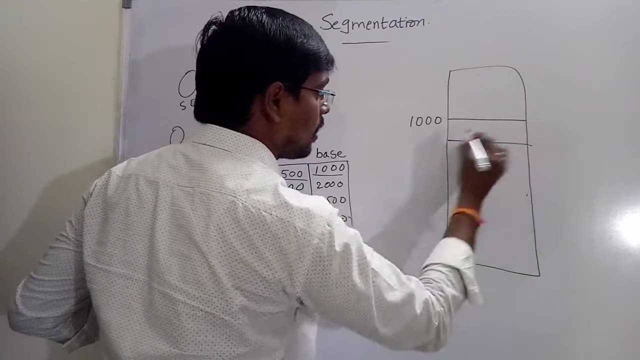 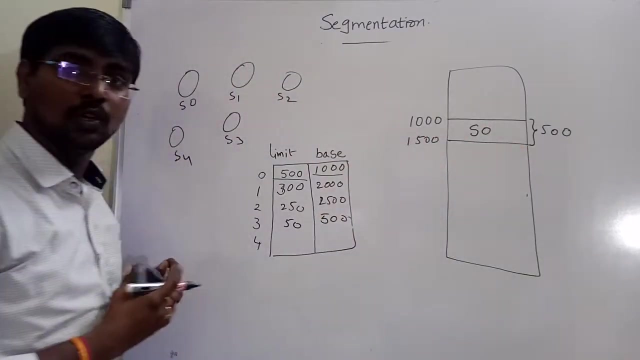 Only 50 At address 1000, Assume this is the address 1000 A 500 elements. This is the size of only 500, That is, 1500. In this position, segment 0 is placed. In this position, segment 0 is placed, Suppose here. my question is: